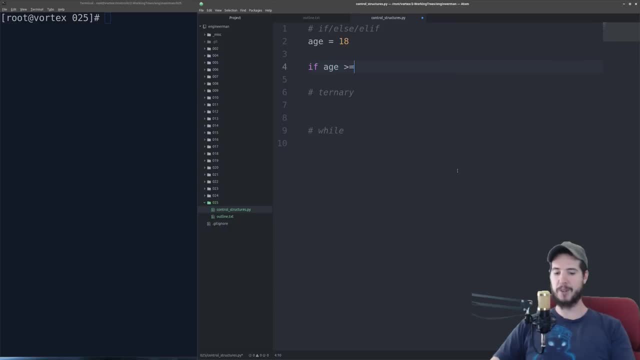 So in this case we would do if age is greater than or equal to 18.. Now at the end you must do a colon And that says you've ended your expression On the next line indented out, You would do something here if age was greater than or equal to 18.. 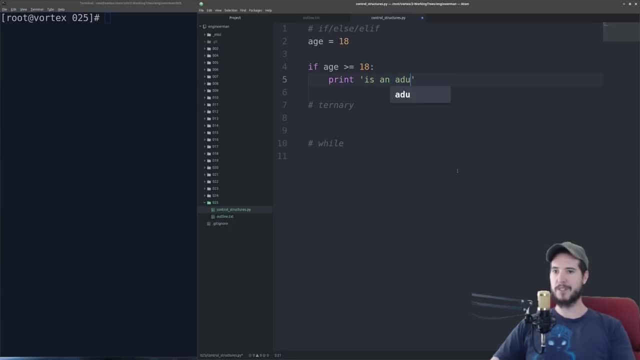 So in this case, we'll simply print isAnAdult. So in this case, the only time it'll print out isAnAdult is if age is set to something that's equal to or greater than 18. If it's 17 or lower, it would simply do nothing. 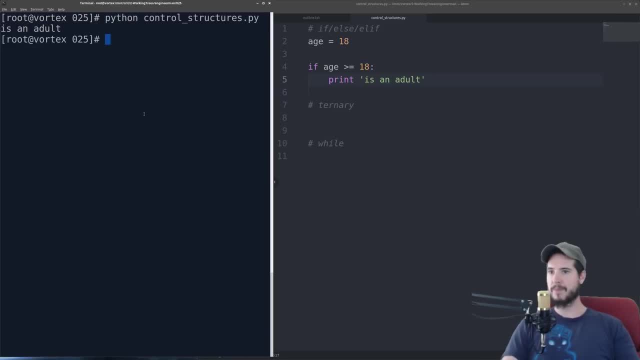 So in this case we could run this program And see that it says isAnAdult. If I change it to 17 and run it, you see nothing happens. So in this case we could run this program and see that it says isAnAdult. If I change it to 17 and run it, you see nothing happens. 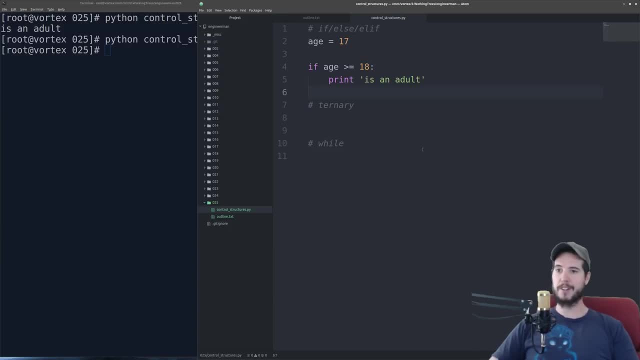 So imagine now you want to perform some action if they are not an adult. So we'll do something simple. This is where the else comes in, Else colon and then again indent. We'll just do the opposite. Print notAnAdult. 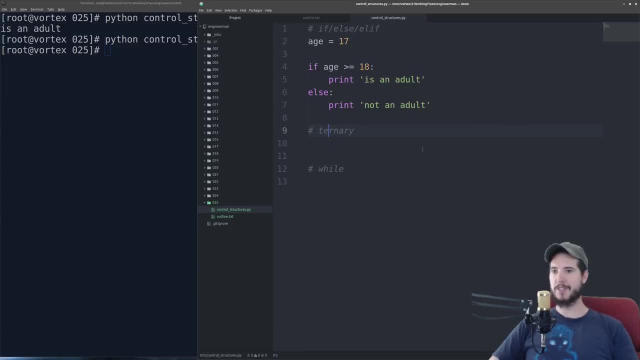 So what this does is, if age is set to 17 or less, it's going to print out notAnAdult, And if age is set to 18 or more, then it's going to print isAnAdult, And we can see that that works. 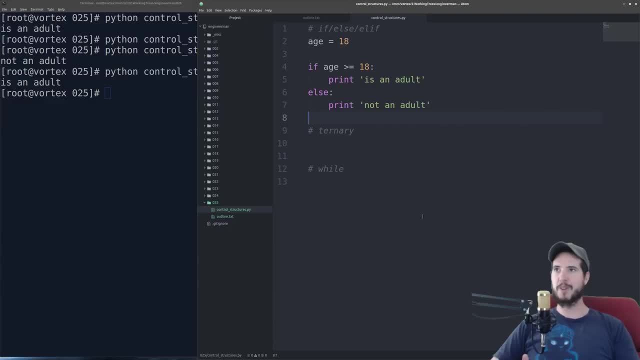 Over here. So imagine now you want to write a piece of code that checks a number of ages. Perhaps you want to check if somebody is an adult, if they're a young adult, if they're a child or if they're, we'll say, a baby. 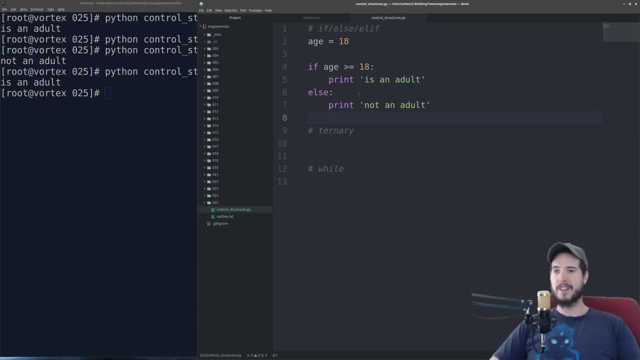 So this is where elseif comes in. So right now we have the check from age greater than or equal to 18.. But now let's check greater than or equal to 12.. So we would do lif, which is short for elseif. 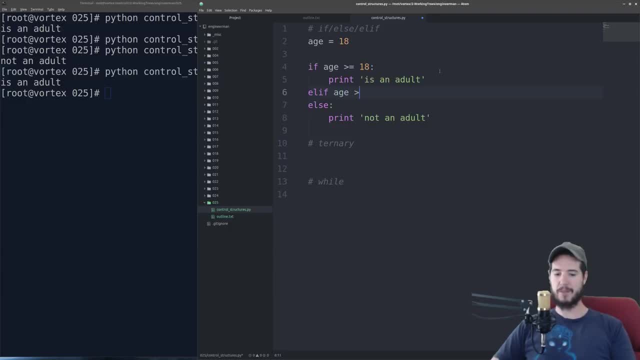 And then we would do elseif. And then the expression Age greater than or equal to 12.. So here we'll simply print: is a young adult, And we can add as many as we want, Because if one of these conditions evaluates to true, it's simply going to run this. 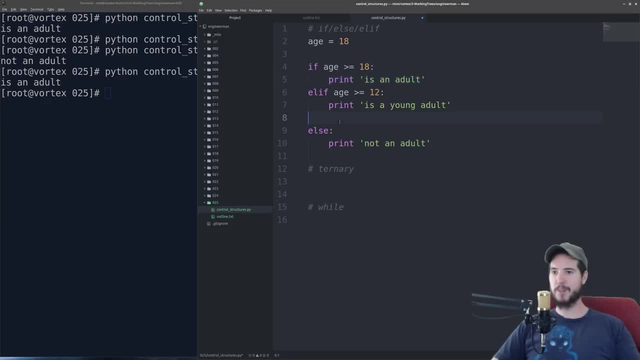 It's not even going to check this next one or go into the else block, So we'll add a couple more. lif age is greater than or equal to 3.. In this case, print child. Now we do have to change the else. Because 18 or over is an adult, Equal to or greater than 12, but less than 18 is a young adult. Then equal to or greater than 3, but less than 12 is a child. Everything else is a baby. 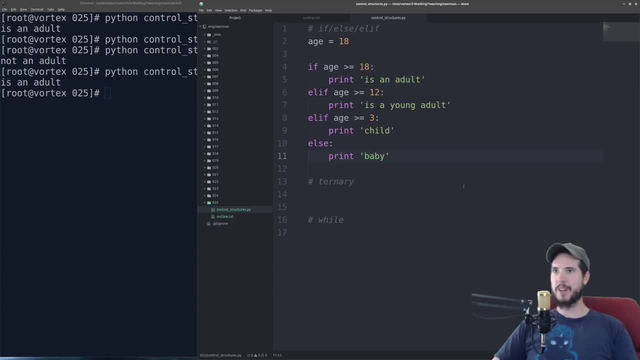 Next is the ternary if. Ternary if is a short way of writing an if statement. So consider a simple piece of code like this: If age is greater than or equal to 21,, then old enough equals true. Else old enough equals false. 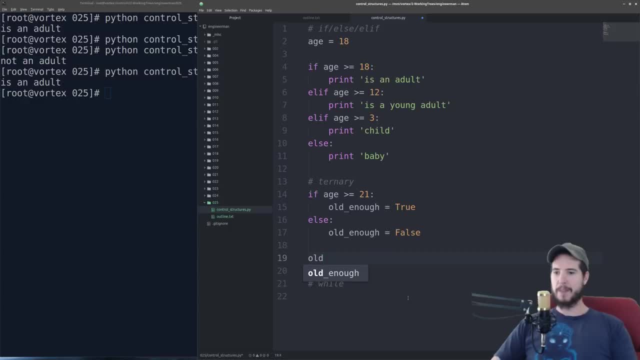 So there's an alternative way to write this. You can simply do old enough equals, And then the way the ternary works is: you have the thing to execute if true, The condition And the thing to execute if false. So imagine this: 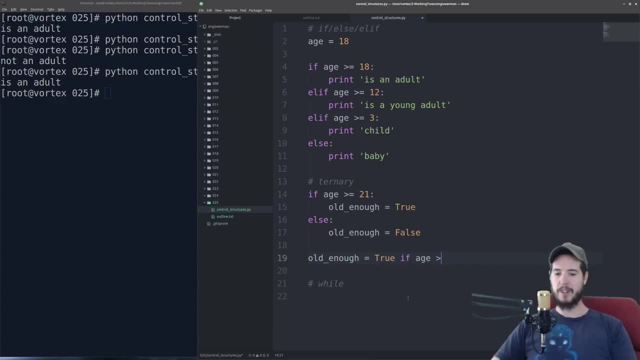 True if age greater than or equal to 21,. else false. So old enough will either be true or false, based on the age In the middle. here is the condition. This is what to set it to if true. This is what to set it to if false. 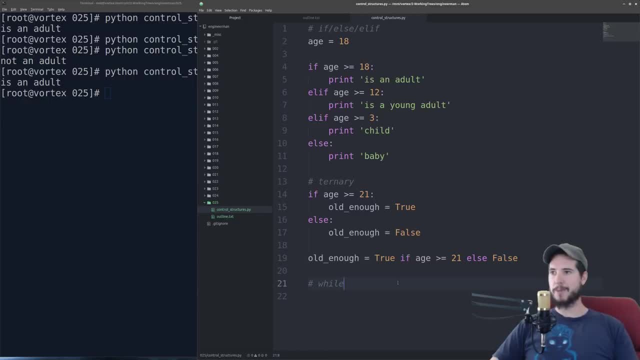 Last is the while loop. What the while loop is for is to execute code over and over again until something, until the expression evaluates to true, So you would do while And then, after while, you would do the expression. So in this case we'll do age less than 50.. 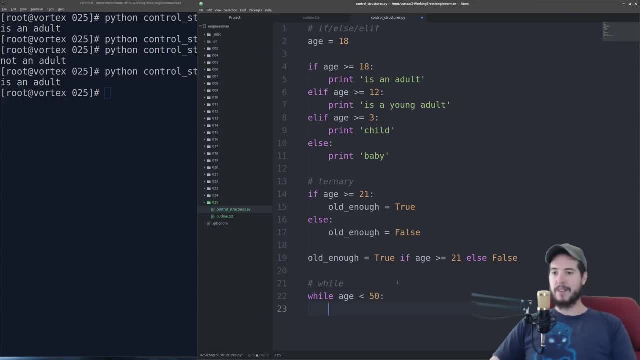 So everything that comes to mind Comes after the while loop is going to get executed over and, over and over again as long as age is less than 50. So, of course, if you never increment age and age is always less than 50, it's just going to be an infinite loop. 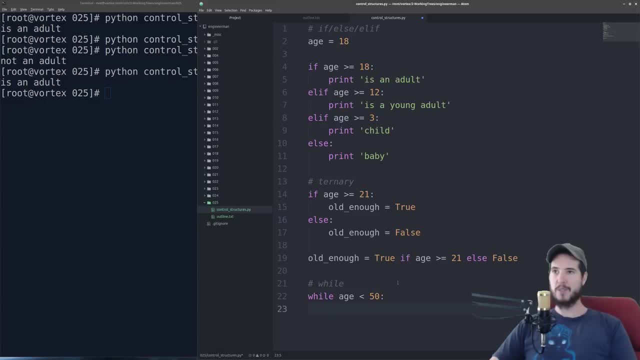 It's going to just run over and over and over again. So what we'll do is we'll print out: say not old enough. Then after that we're going to increase age by one. And now what this will do is it will execute over and over again. 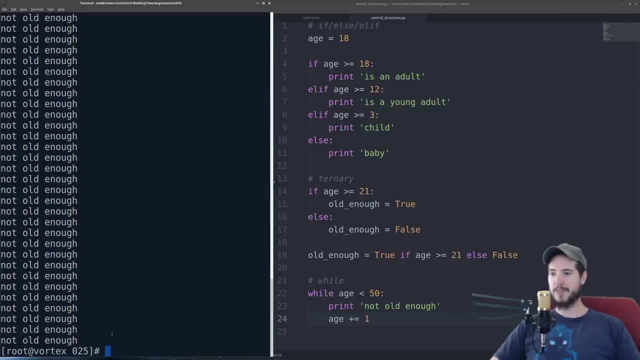 See it here. You can see it executes a bunch of times And then it leaves And it executes exactly 50 minus 18 times, So 32 times, And we can visualize this by you know, not old enough. current age is age. 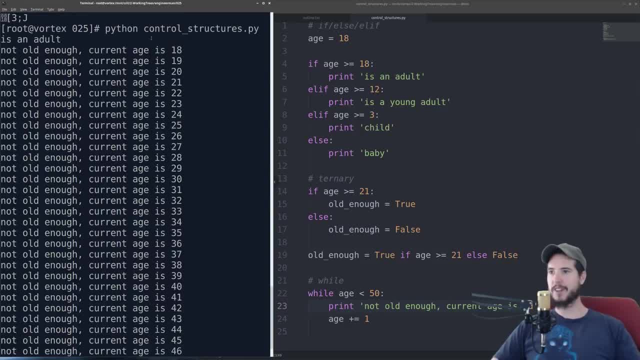 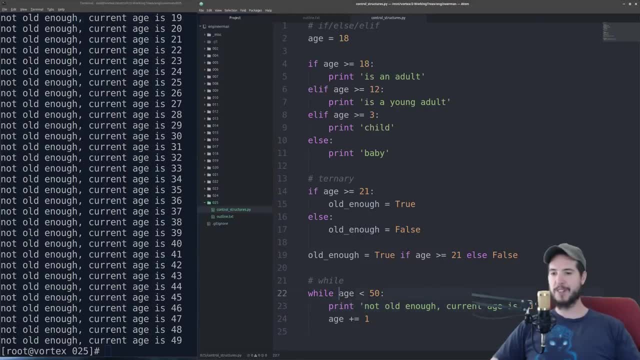 Now we run it again. See, not old enough. current age is 18,, 19,, 20,, all the way up to 49. And you see, once it got to 50, age became 50. And it said: while age is less than 50..